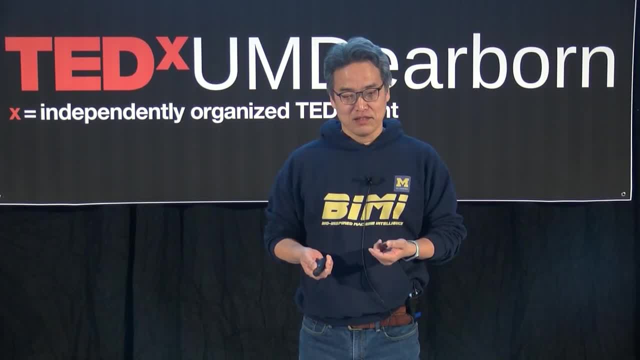 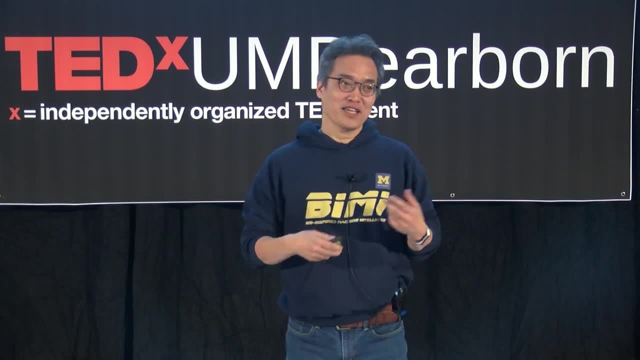 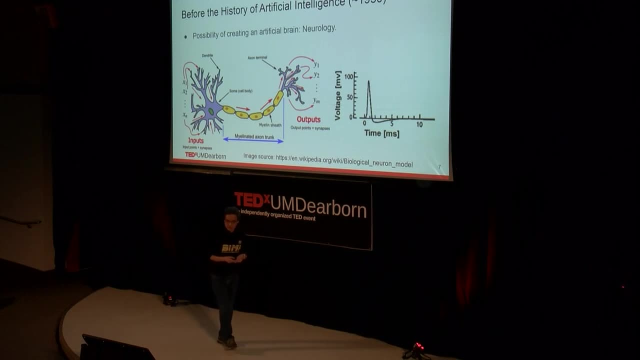 and then change internal state. That was the first ever like a computer that can do something other than just calculation. And in 1950, in urology, researchers found out: a neuron sends signal to another neuron through just high volt or no volts, okay, Which means 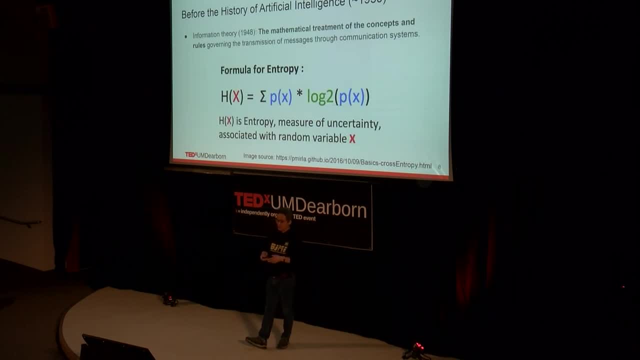 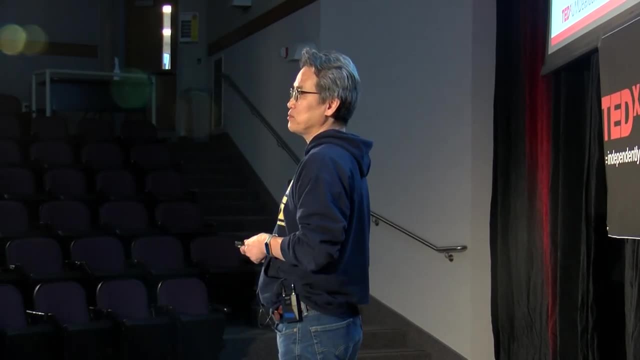 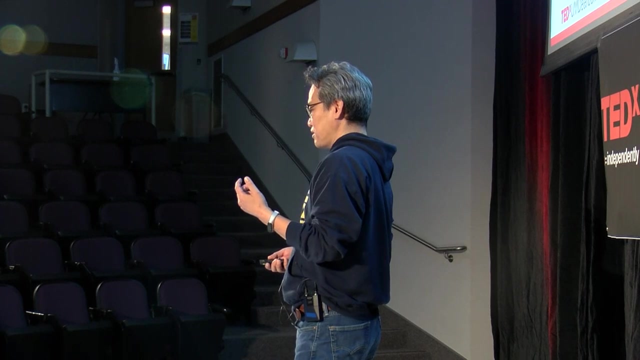 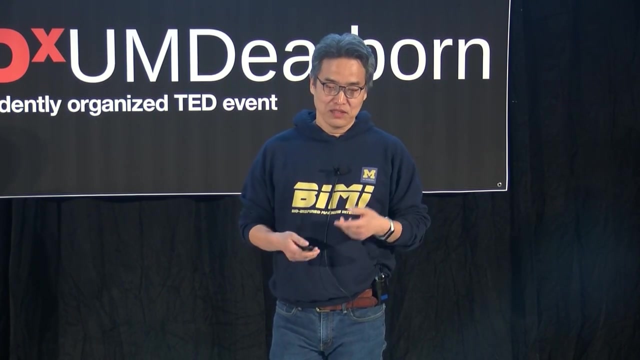 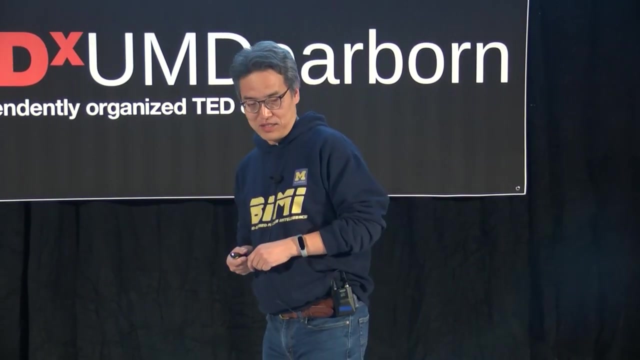 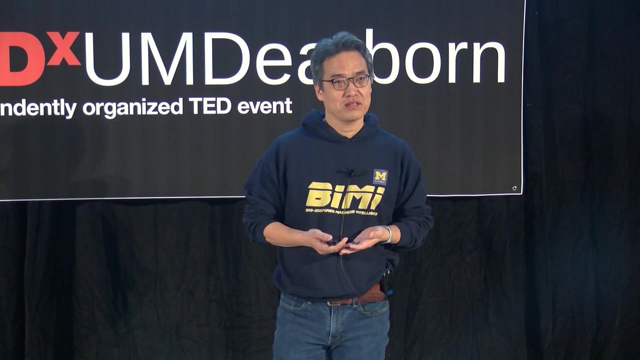 basically a binary signal And information theory established by Cloud Shannon. He's one of our, you know, alumni, University of Michigan- And the important point of this information theory is now: your concept can be expressed by a mathematical term And in 1943, Macar and Pitts proposed the first ever mathematical model of artificial. 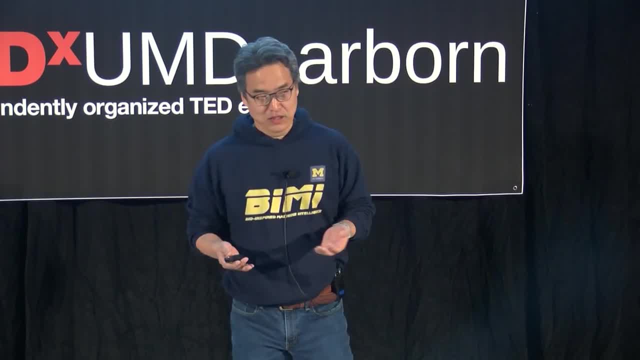 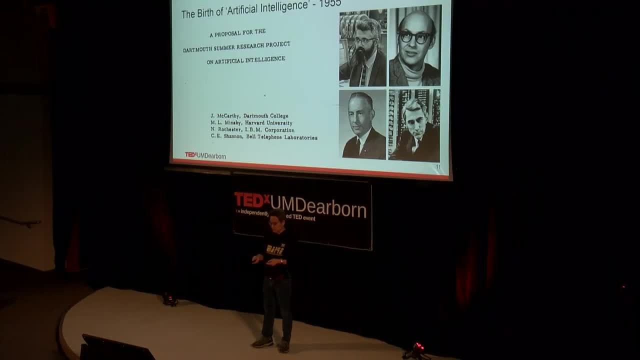 neural network And thanks to these advancements, in 1955, John McCarthy and Marvin Minsky and Rochester and Shannon proposed some research process for neural network And in thisлеans, aerospace theory, I would like to present a collaboration And we have actually 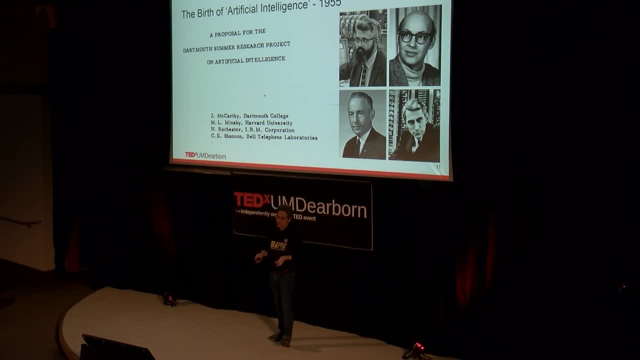 of course, several guests today… And within thejohn and me, I'd like to talk about what the on artificial intelligence. why this is important? because the name artificial intelligence was coined by Marvin Minsky in 1955, the first ever. it's weird to. 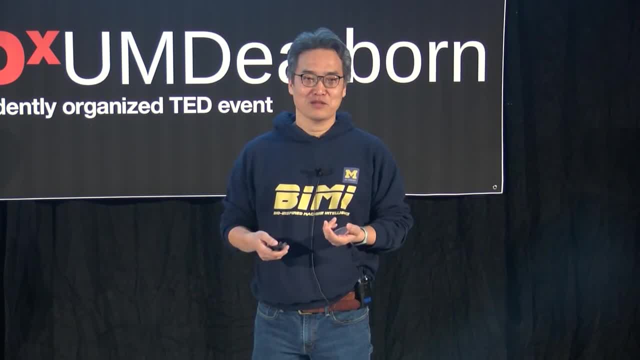 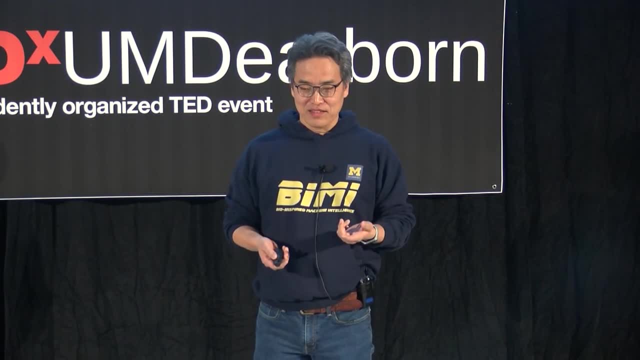 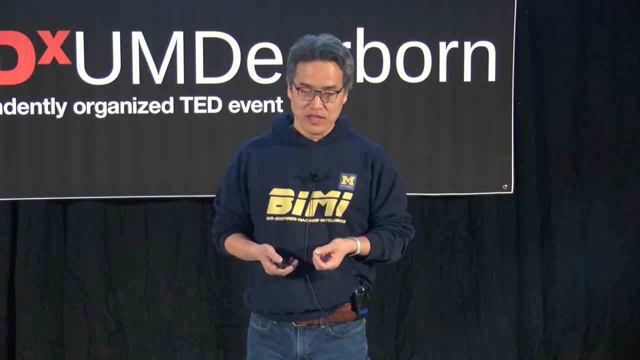 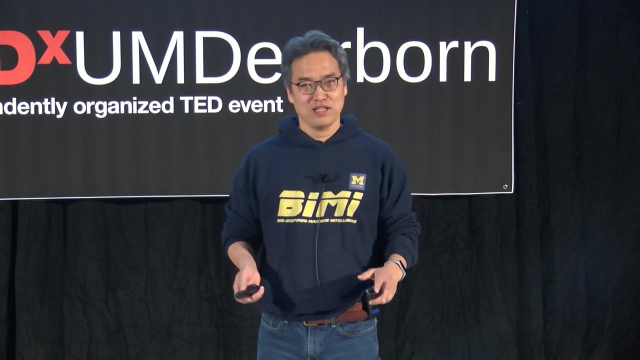 think about intelligence. intelligence is very unique to human beings, right. and what is then artificial intelligence, right? so from then, 1956 to 1954- I mean 74- we had intense optimism. we also called the golden years. quote: every aspect of learning. intelligence can be so precisely described that machine can. 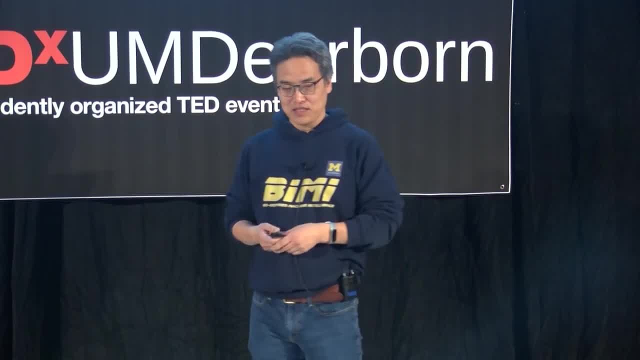 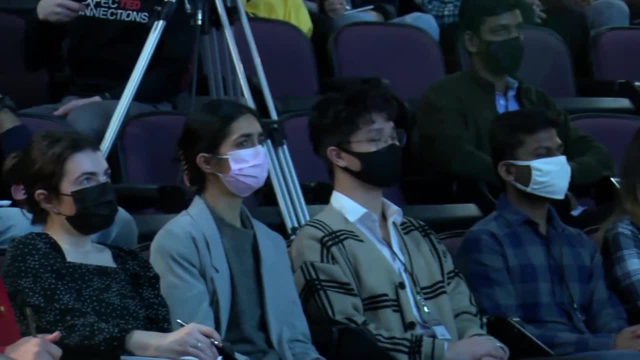 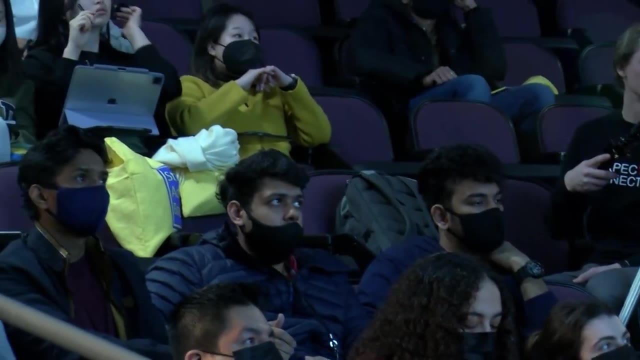 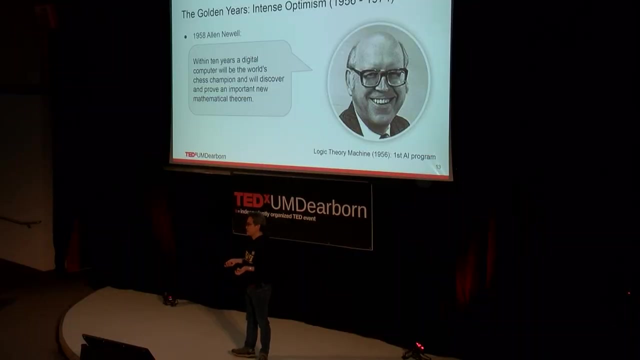 be made to simulate it. so in 1958, Alan you are. he was the first AI program writer. quote: within 10 years, a digital computer will be the world chess champion and will discover and prove an important new mathematical theorem. what really happened in, I believe, 19, 19, 8 or 19 708 actually? after 40 years later, we had a. 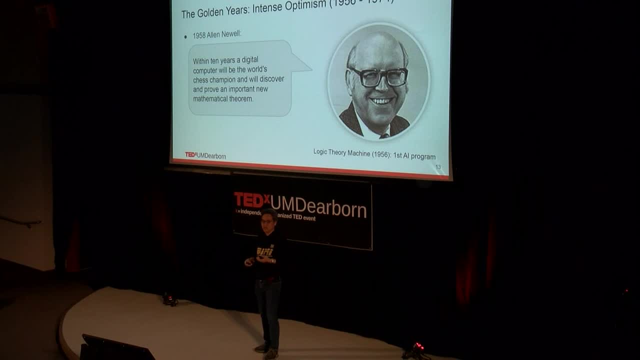 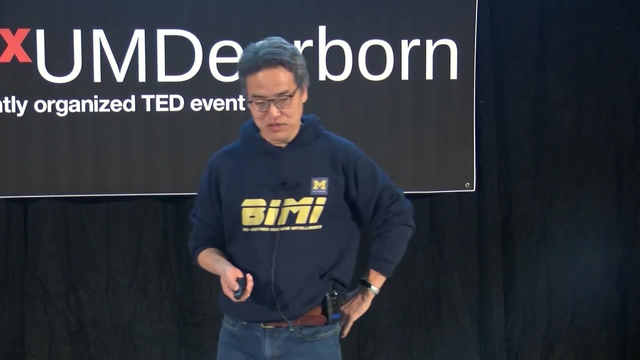 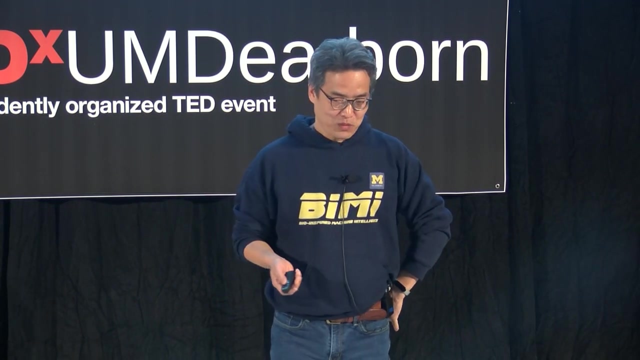 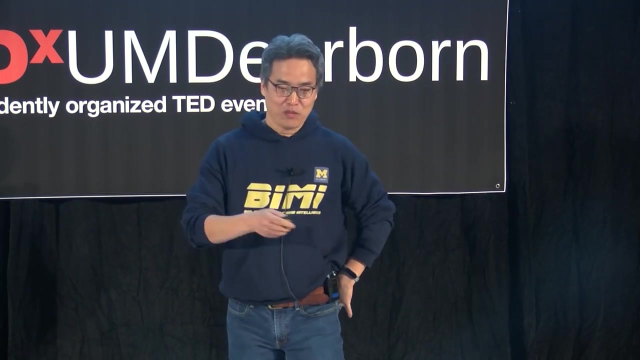 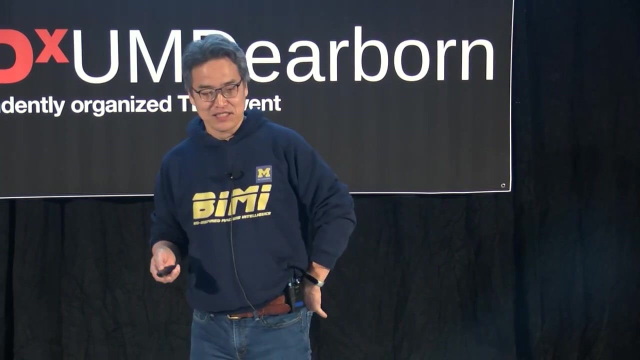 IBM Big Blue specially designed expert system to play chess. and in 1965, Herbert Simon. he's a pioneer of RA, artificial intelligence. quote: machine will be capable within 20 years of doing any work a man can do. Think about: this is 65,, okay, 20 years later, 85,. never happened In 1967,. 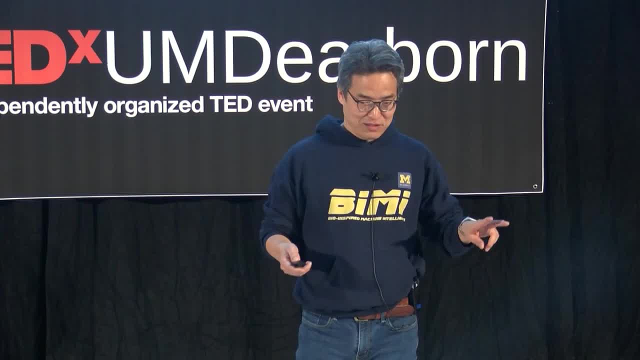 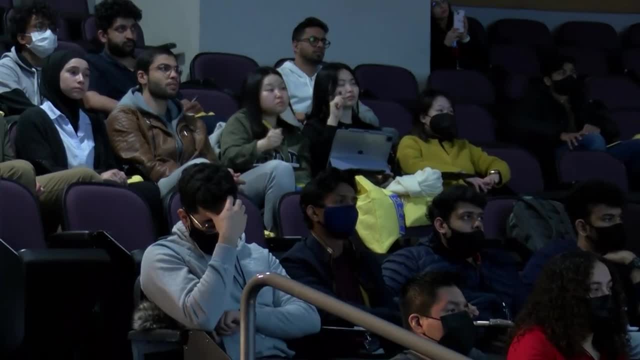 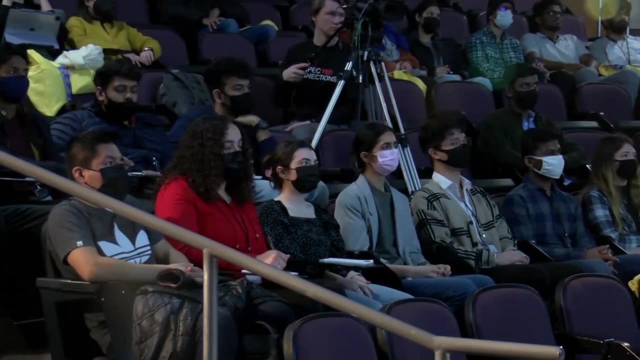 Marvin Minsky said, quote: within a generation, 30 years, the problem of creating artificial intelligence will substantially be solved. And in 1970, he also said, quote in from two to eight years- we will have a machine with the general intelligence of average human. 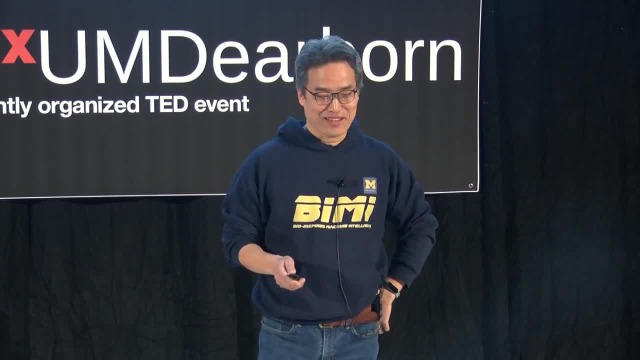 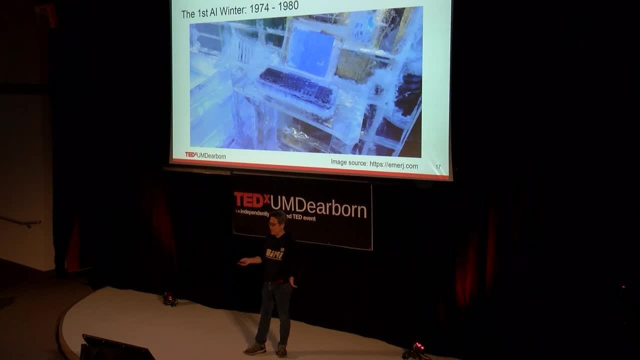 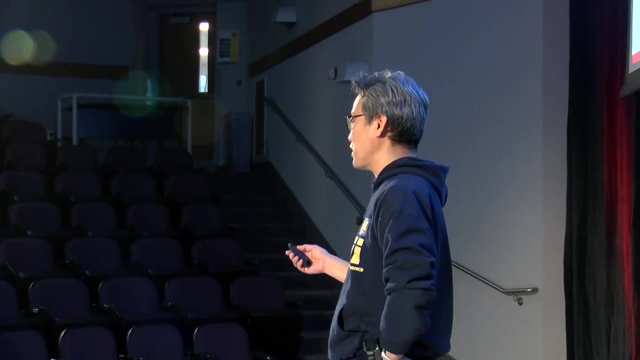 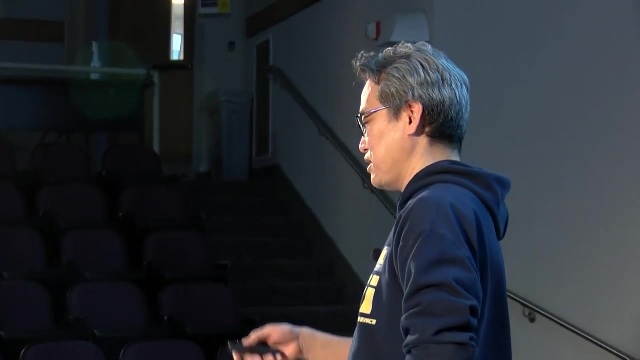 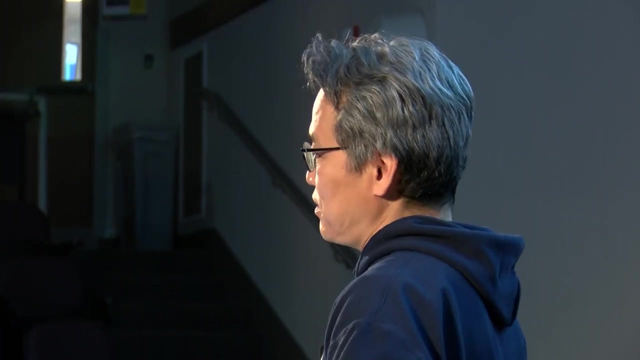 being That was 1970. Okay, remember that. Then what We had? our first AI winter from 1974 until 1980. Because the government. We had a short rise from 1980 to 1987, thanks to an introduction of hidden neurons, and then 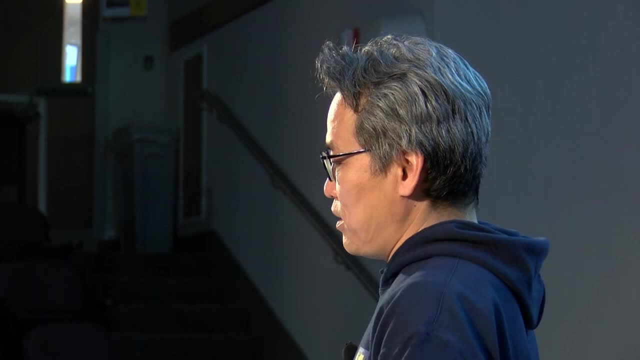 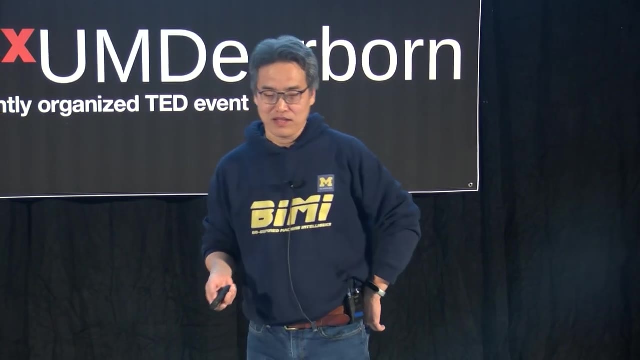 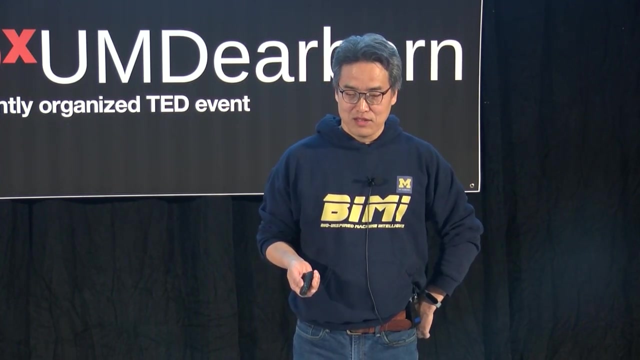 the learning mechanism back propagation. But we had a second AI winter from 1980 to 1987 to 1998.. And then, disguised, from 1993 to 2011.. During this time people didn't want to say their techniques AI-related. Rather they say: 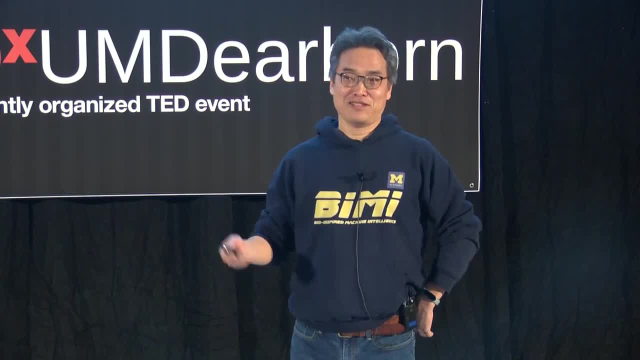 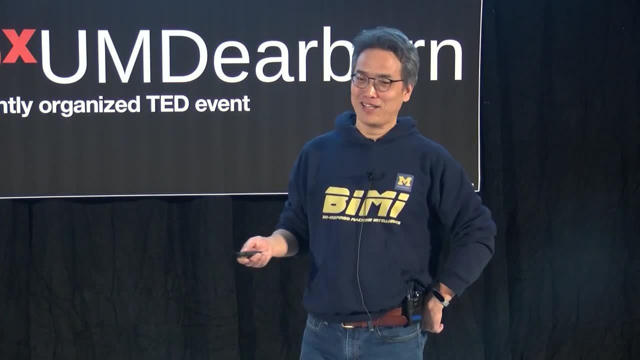 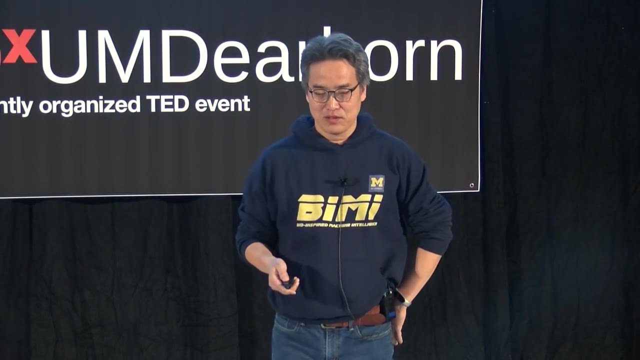 oh, this is character recognition, or this is intelligent agent, Or this is machine translation, or this is computer vision or robot vision, Because the name was so tainted. And what happened in 2011, or more precisely, 2012,. until now, 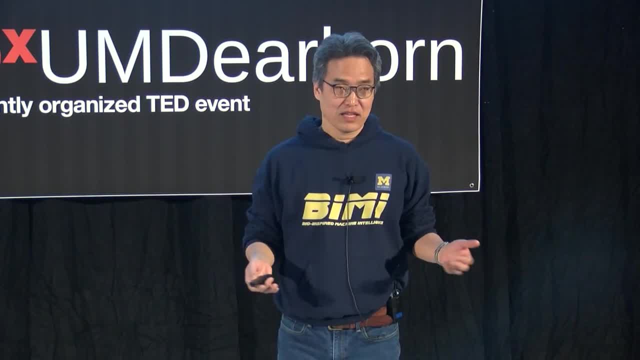 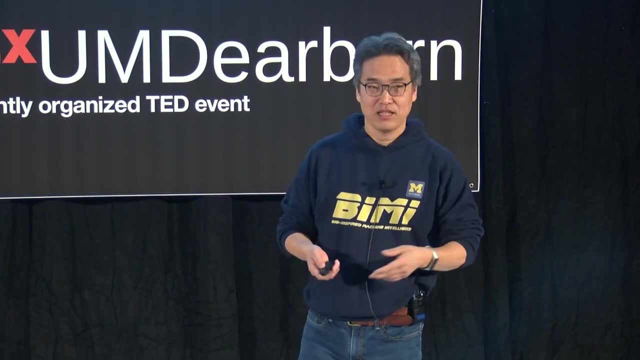 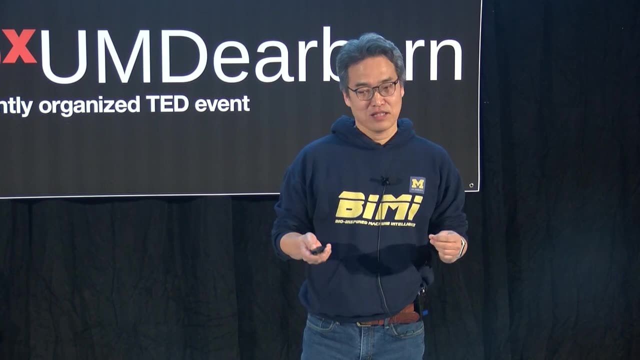 we had a large amount of data thanks to your mobile phones, and then GPU, that's the computing, parallel processing, and then new deep learning techniques. This is a tipping point for this deep learning Big Bang. That was 2012.. 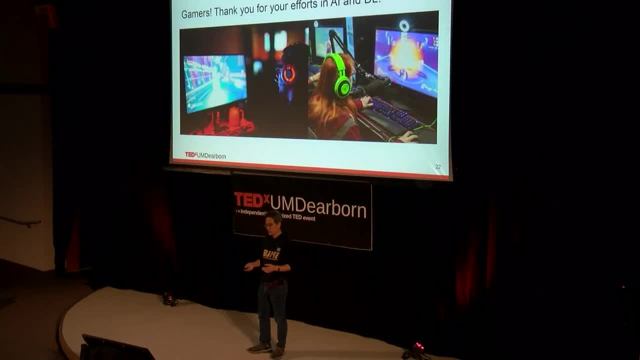 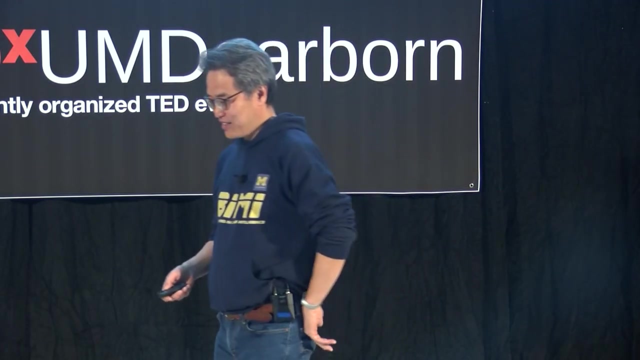 Gamers, thank you for your hard work for AI and machine learning, including my sons. Without them, it wouldn't be possible, So I really, really appreciate your money and time, And then we can discuss AI challenges for connected autonomous vehicles. 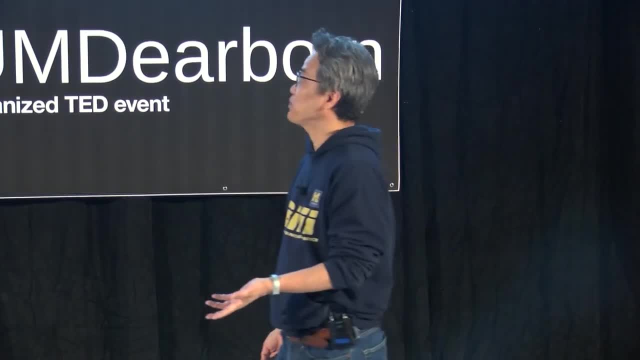 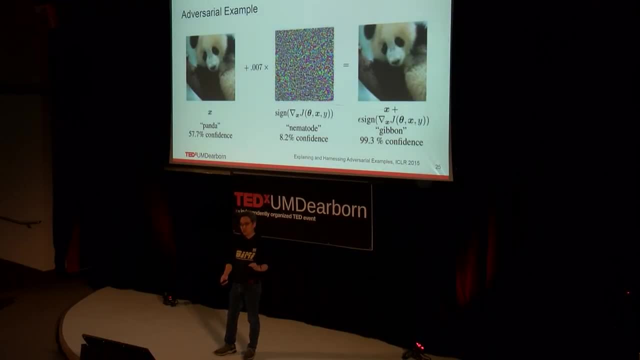 First adversarial attack. Well, adversarial attack is an example. The left side, It's a panda with a 57.7% confidence By simply adding noise to this image. and the right side is almost identical image but with some noise. 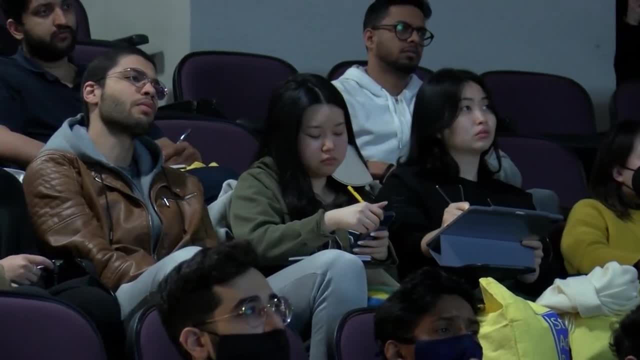 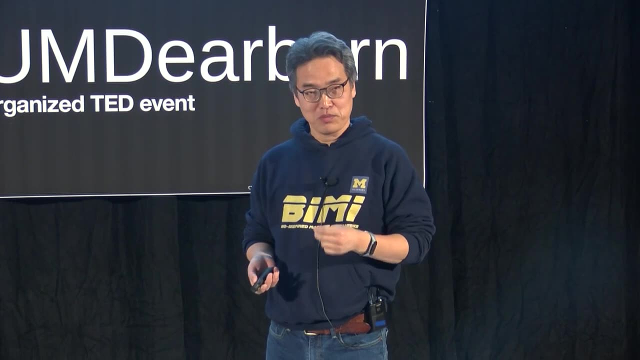 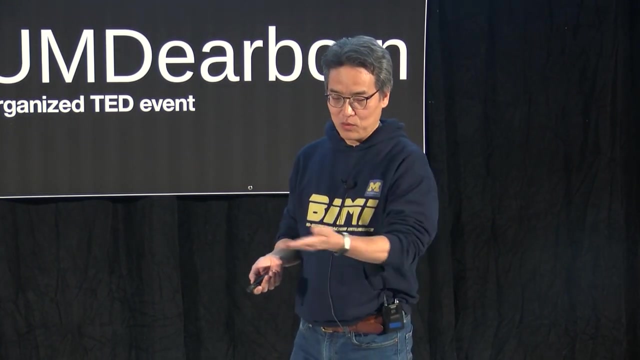 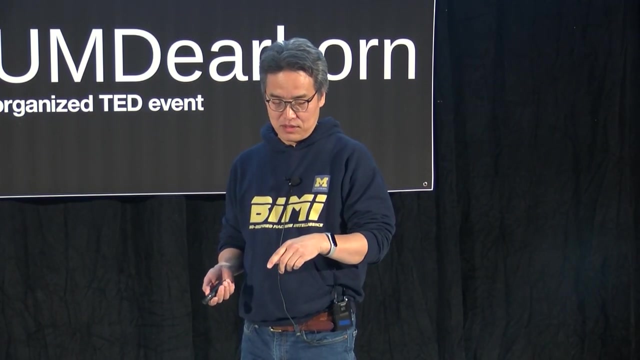 But if we put this panda image to the same system to classify what this object is, we have a 99.3% confidence, given monkey. And the second example is: these are all stop signs. We have some camouflage, graffiti or the tapes. And since, even though these are all stop signs, 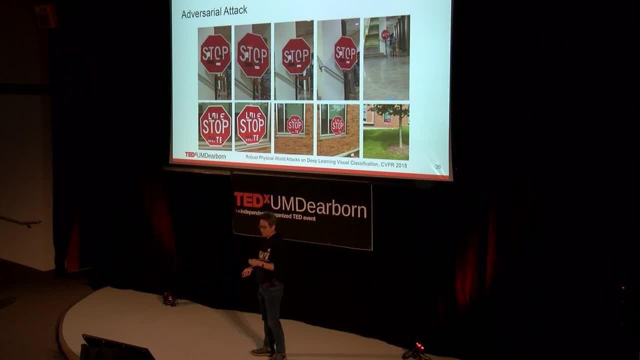 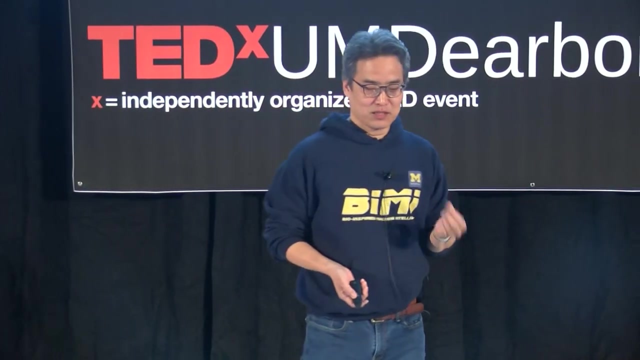 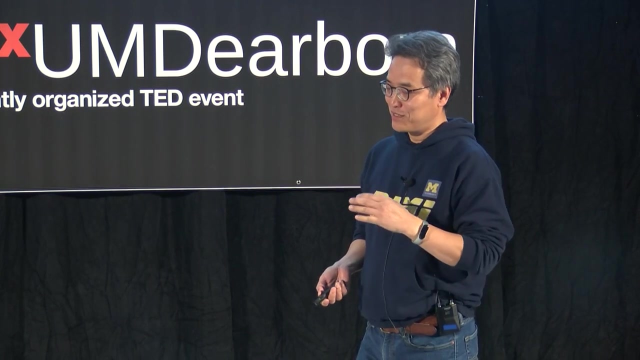 but the original stop sign classification AI system classify these as limit speed limit, 45 miles or yield sign. So the second challenge is a explainable artificial intelligence, or CHI In 19,. no, it's not 19.. OK, 2016,, there was a game with this AlphaGo. 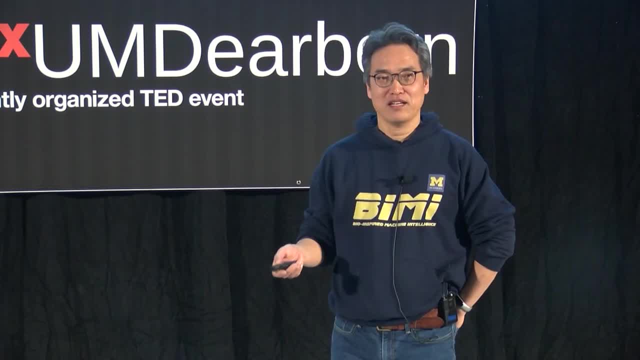 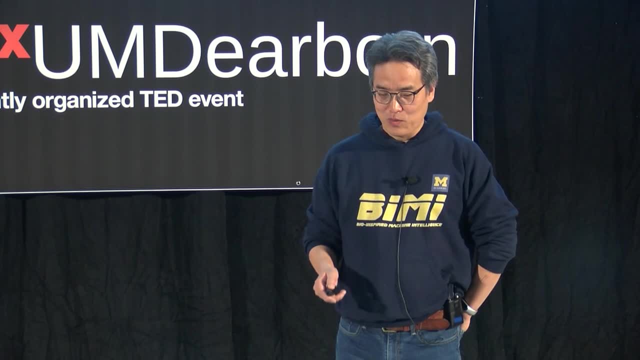 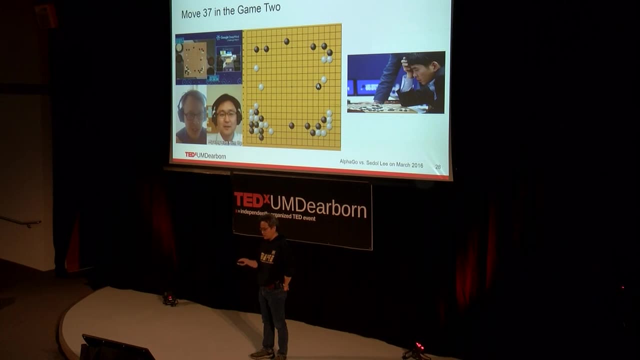 And Sedol Lee was a Naingdan Go player. There was a move 37 in the game too, When AlphaGo put that stone in the game, that stone there. no one understood, including Sedol Lee, including these commentators. 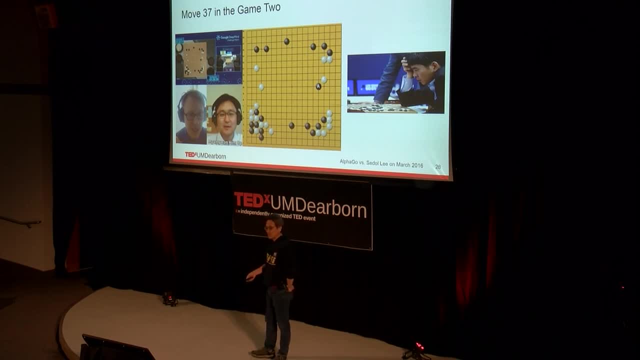 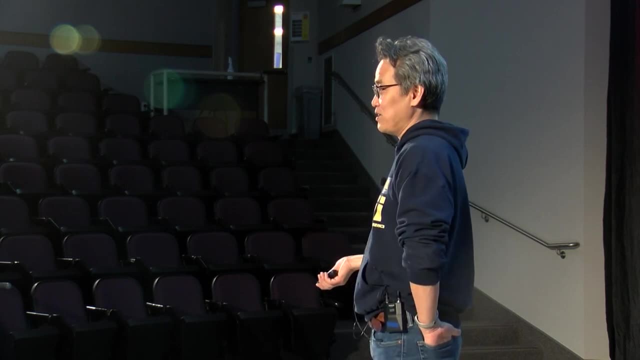 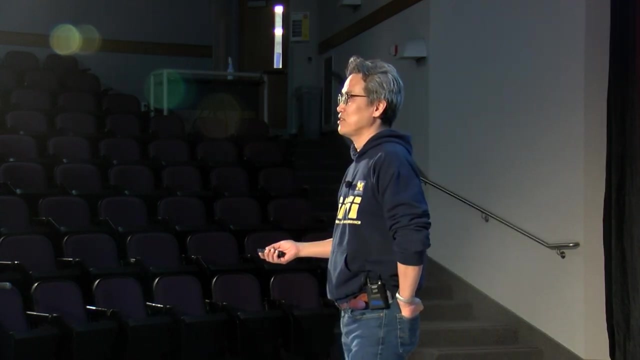 No one knows why AlphaGo did that, But it turned out. this is really important. And then it changes the course of the game. It can be OK, not understanding why this AlphaGo did that, But what if nuclear reactors? If you have an AI system, it has mounting evidence. 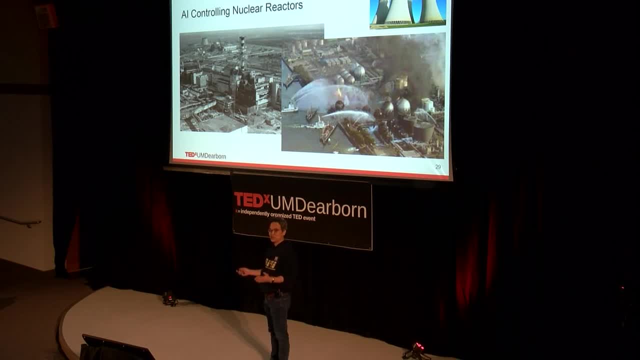 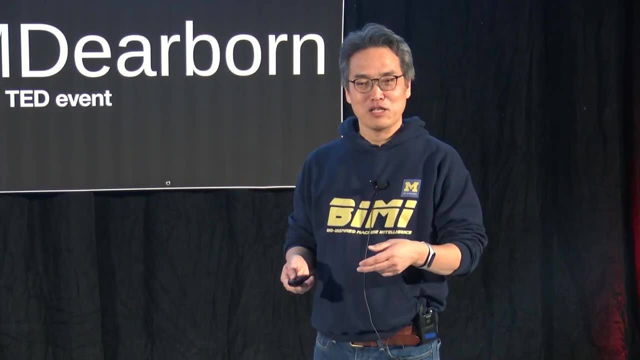 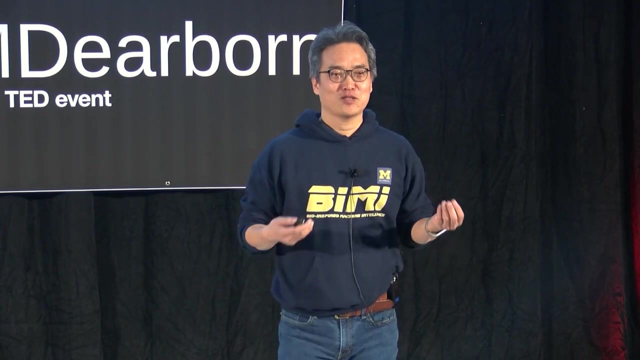 that was really, really good. And then one day it analyzed tons of data and recommends: human operator- hey, something is wrong, do this, But to the human being that recommendation doesn't make sense. Then question is: should we follow AI decision or not? 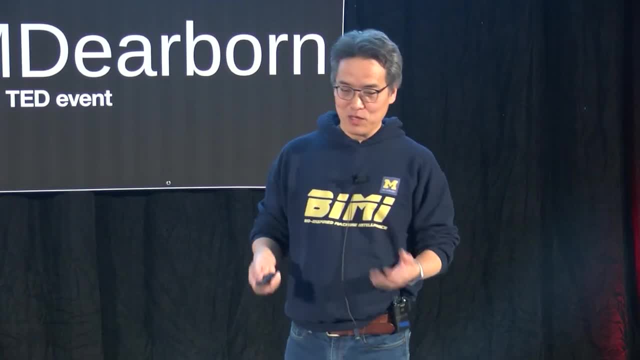 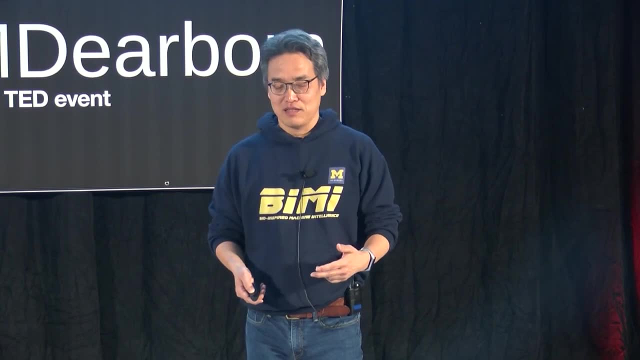 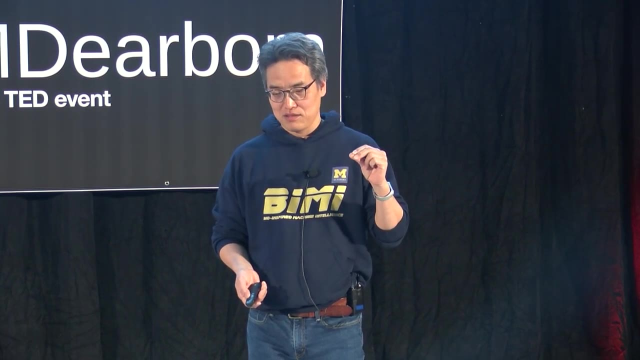 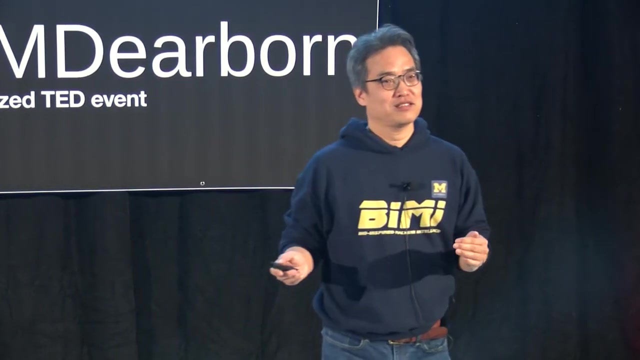 Right, interesting question, right. So explainable AI or CHI means we need to understand more how the AI system makes decisions. But problem is the learning performance will be decreasing as explainability increases. OK, It's obvious, right, We understand better, then problem should be easier, right? 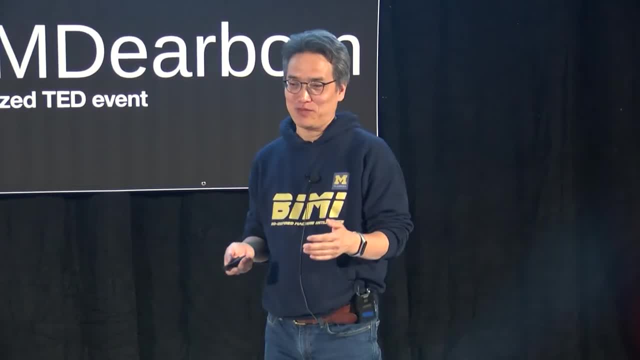 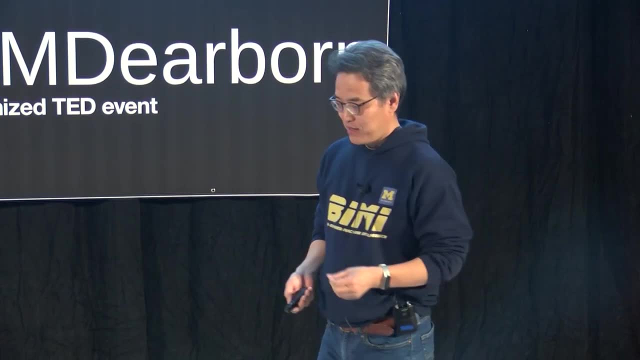 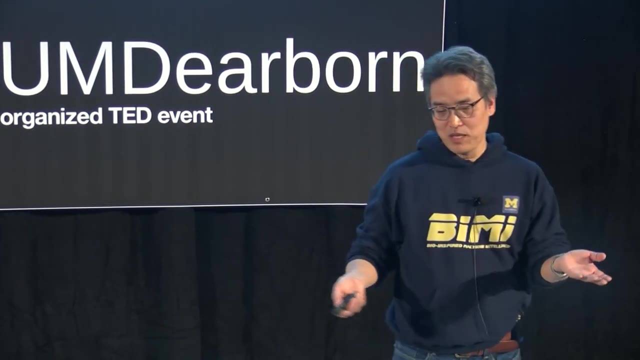 If things really complex, then it's hard to explain, right? So again, there is no answer for now. It's an active research area. And then the third one is machine decisionality. So everybody knows maybe this one, Isaac Asimov. 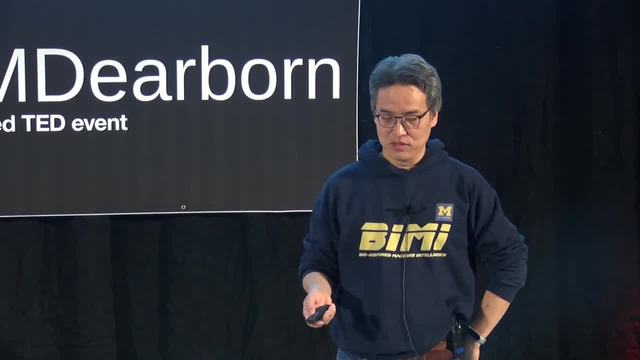 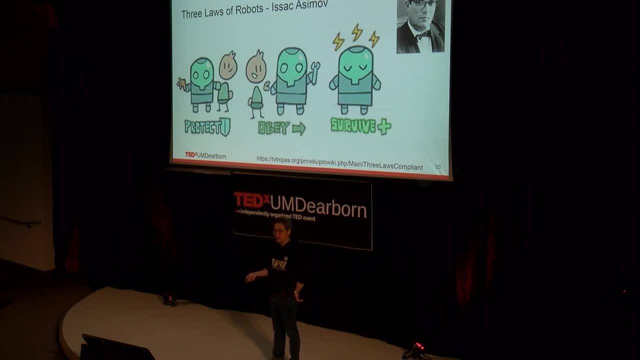 He's a sci-fi writer. Three Laws of Robots: Robots must not injure human beings and robots must not injure humans. Robots must obey human beings' order, except the order against the first law. And then, third one robot must maintain his survival. 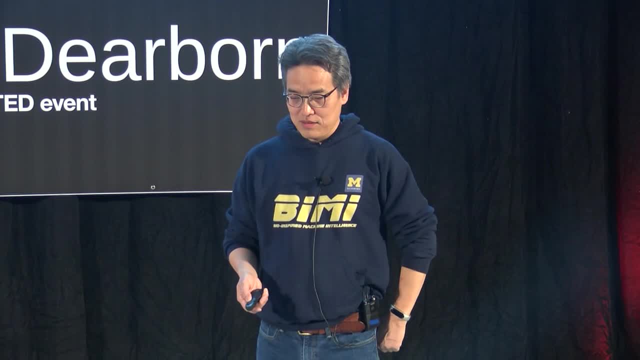 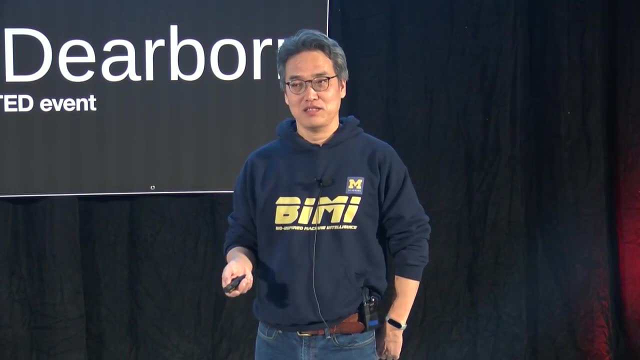 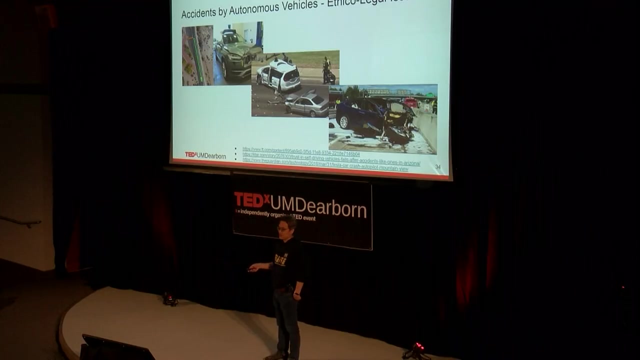 unless like first and second law right. But in autonomous vehicles there are many different cases where these three laws of robots not applied. Like Uber, autonomous vehicle killed a lady who carried a bicycle And then later it found out the Uber AI system. 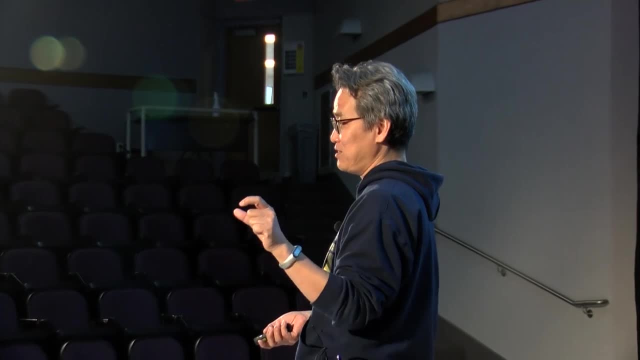 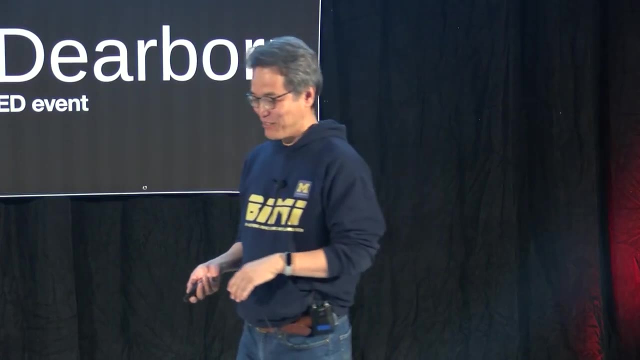 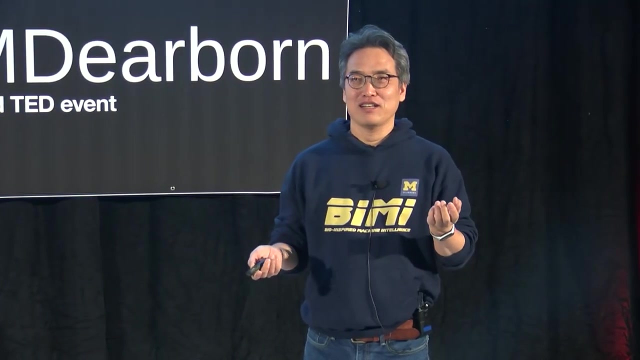 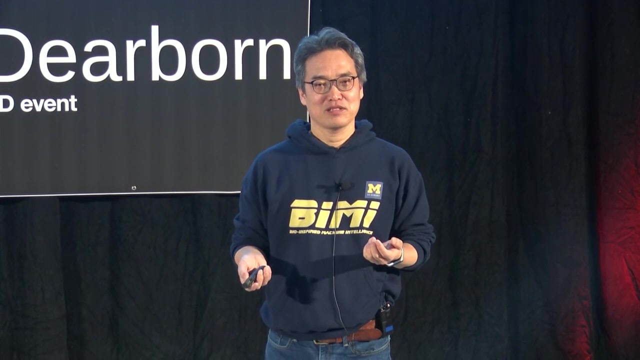 found that object but failed to categorize, So not know what to do. just go. Then You may have a question or you may ask: That was like AI decision and human decision- if they conflict, what we can do. 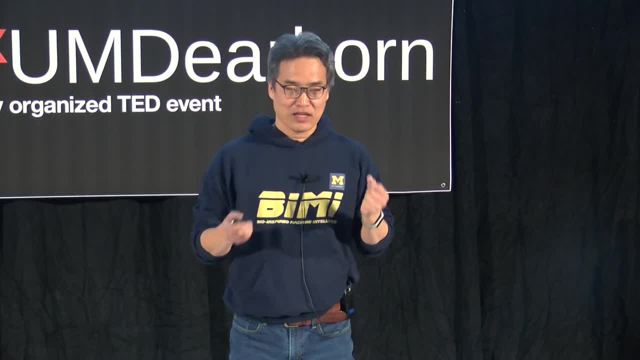 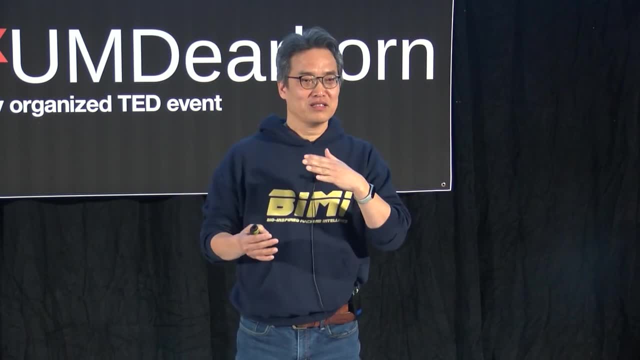 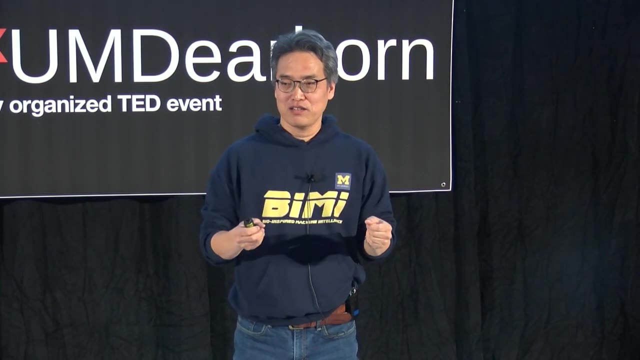 We can ask more complex legal questions. OK, I'm a driver, I'm driving And I lost my attention. AI system knows something is coming And then it's dangerous for that human being. And then I'm the driver, And then I'm the operator. 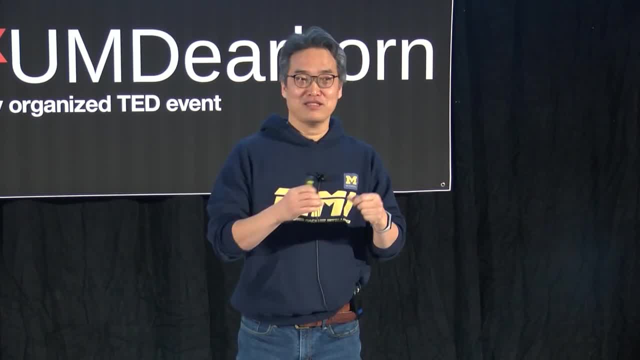 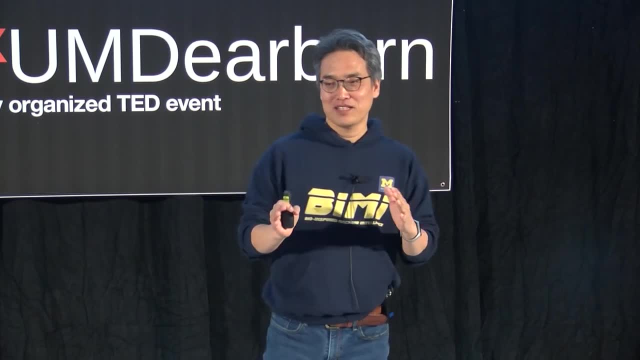 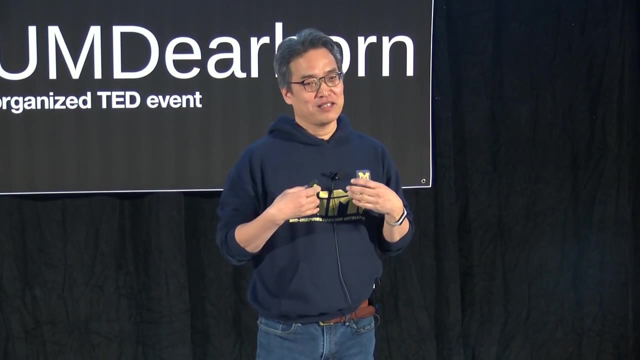 And then I'm the operator, And then I'm the operator, Then AI should override my decision or just kill the human being. It's not as simple as three laws of robots right, Or AI refused my action or my commands. 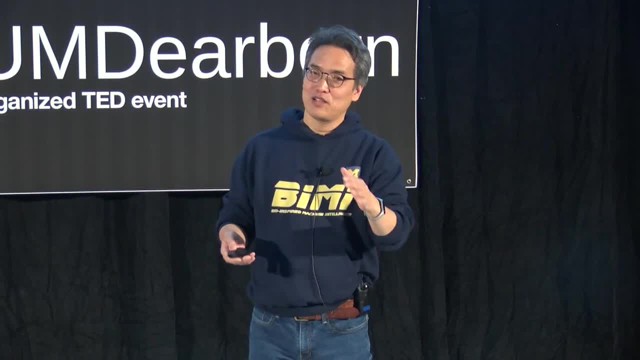 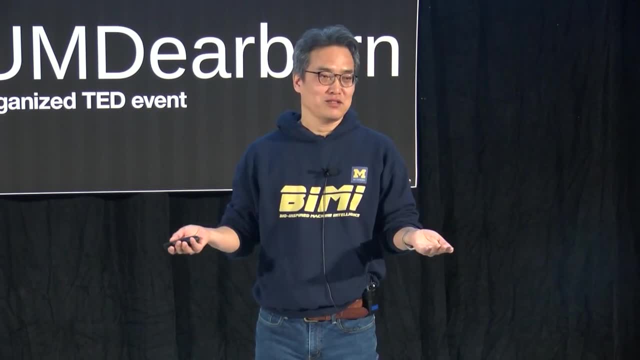 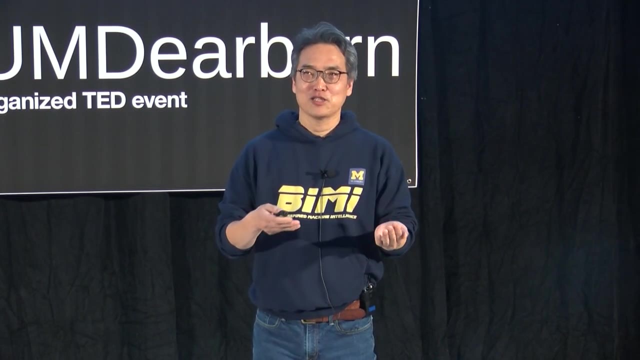 I do this, but AI clearly can think there are possible injury for other human beings. then again, the first law: do not injure a human being. But if your operator say do this, then should AI obey the human being's order. 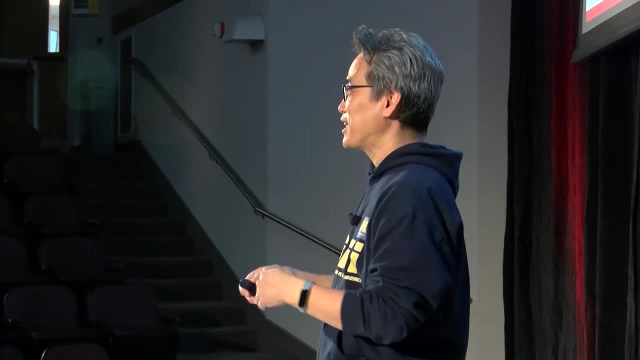 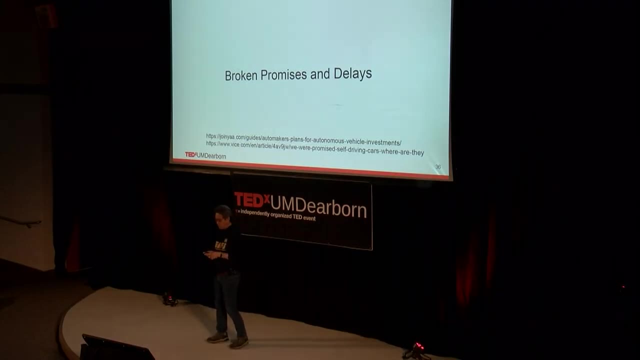 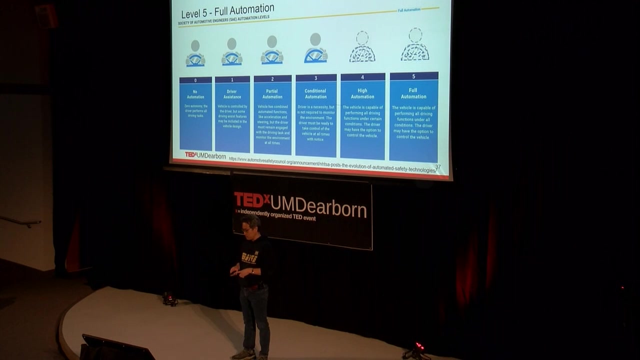 or refuse the order and then save life. No answer for now. right, And before concluding my talk, I want to review broken promises and delays from the automobile industry. This is a level 5 full automation from SAE. The level 5 is full automation meaning. 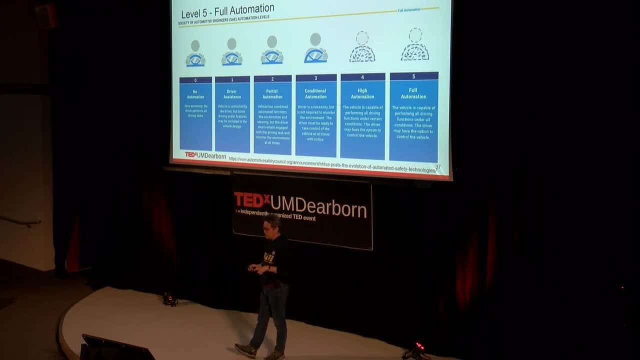 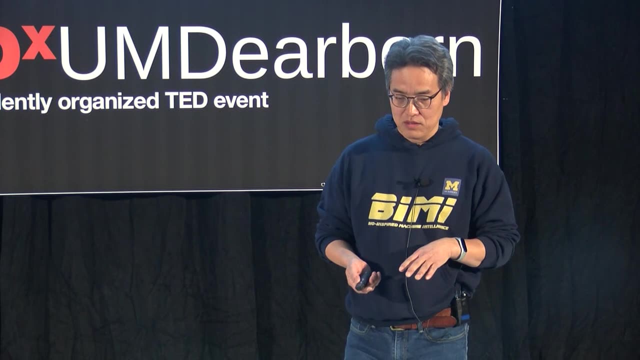 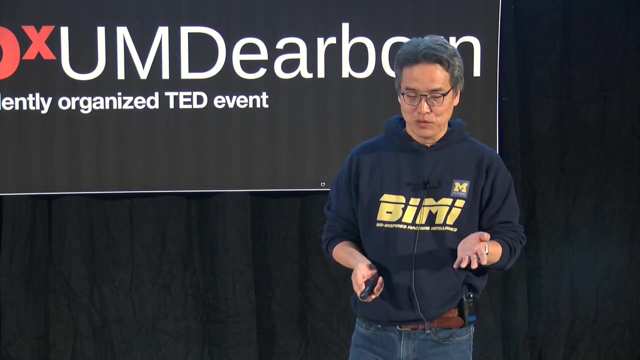 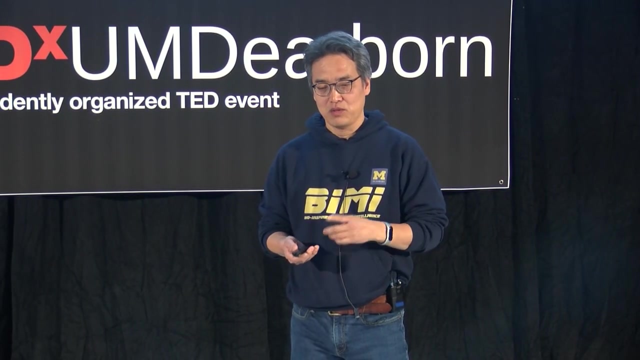 the vehicle is capable of performing all driving functions under all conditions, without exception. So in 2010, there was an intense, intense optimism. similar Ford in 2016 predicted they would have driverless car without steering wheels by 2021.. 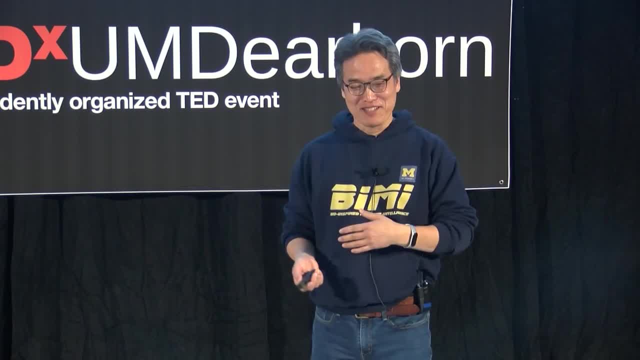 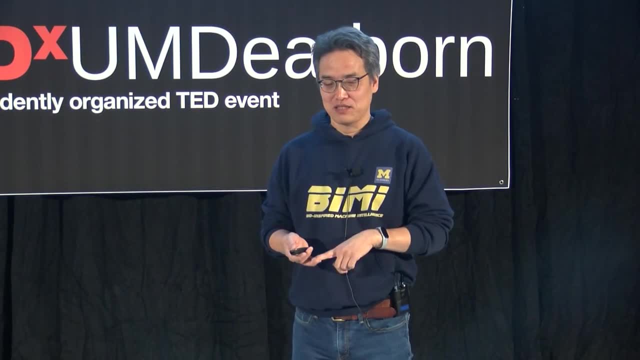 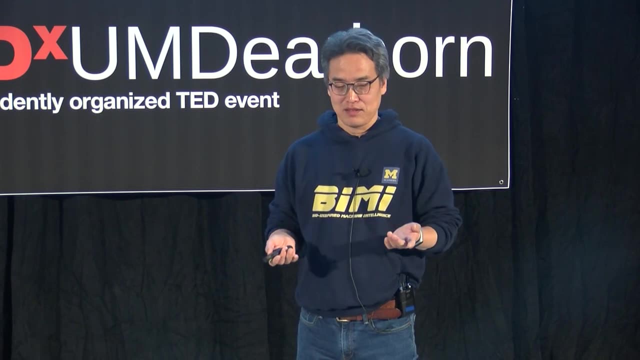 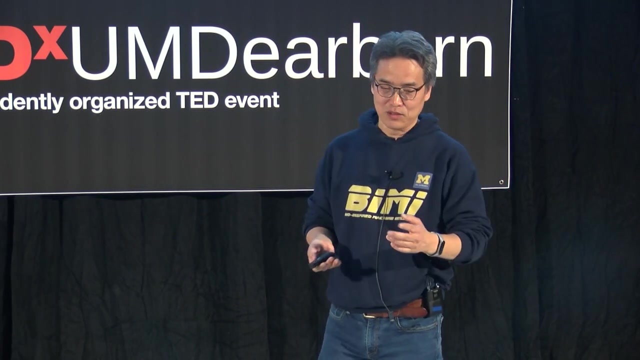 They may say: oh, it's because of the pandemic. good excuse. General Motors has been working on its fleet of driverless Chevy Bolt since it acquired Cruise in 2016.. We don't see this Cruise right, At least here in Detroit. In 2016,. BMW and Volvo also planned to have driverless car by 2021.. The famous guy, Elon Musk, Tesla in 2018, version 9 of FSD means full self-driving would begin rolling out in August. 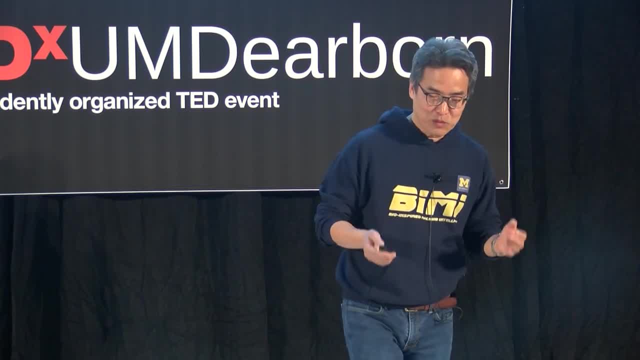 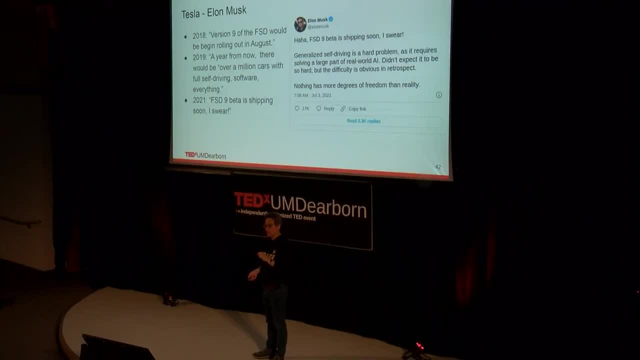 And in 2019, a year from now, there would be over a million cars with full self-driving software, everything In 2021,. last year, FSD 9 beta, now it's beta right, It's shipping soon, I swear. 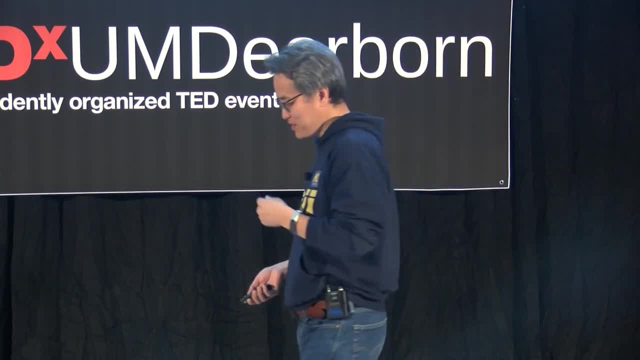 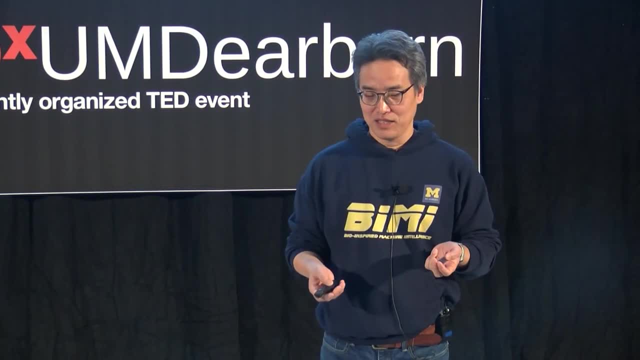 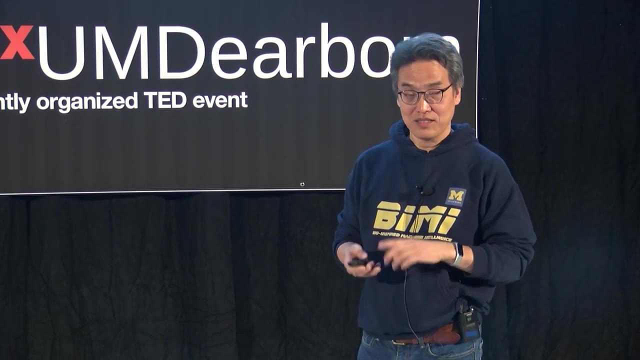 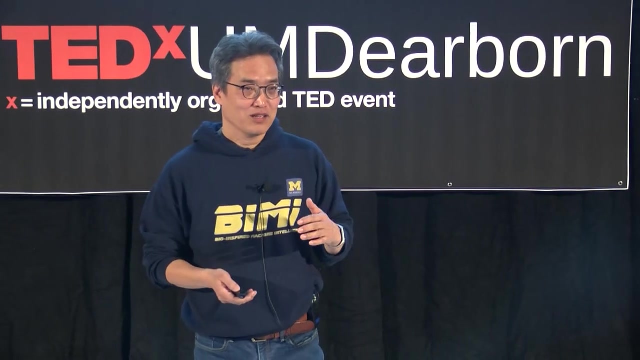 Yeah, there are some similarities, right? So this is my suggestion and conclusion of my talk: To avoid another AI winter in automobile industry, we must accept it is a hard problem And then also we have to accept we are still a long way to go. 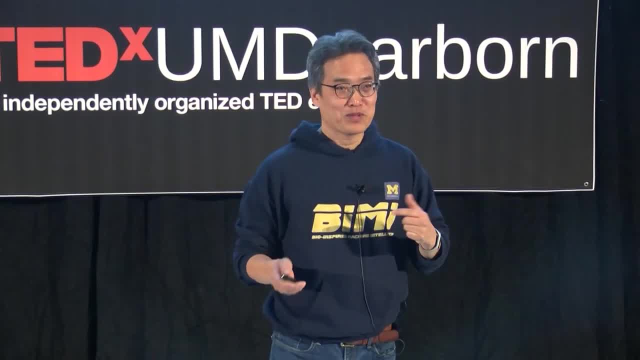 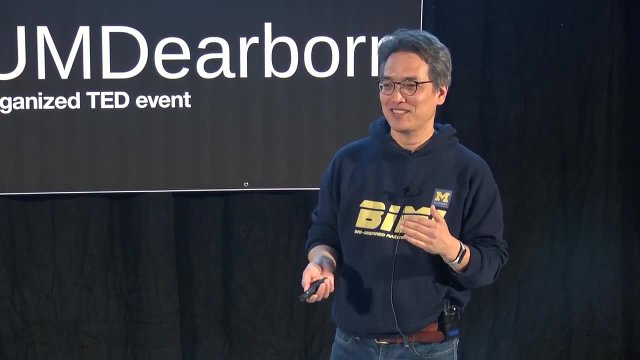 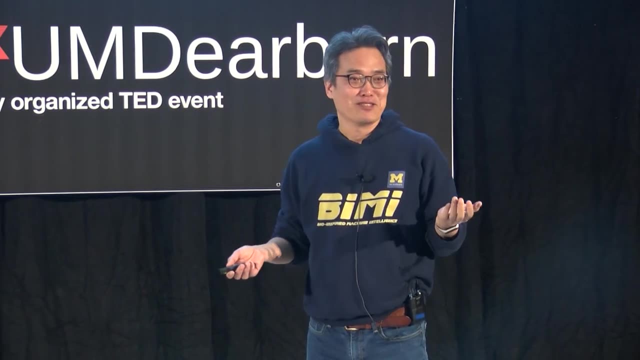 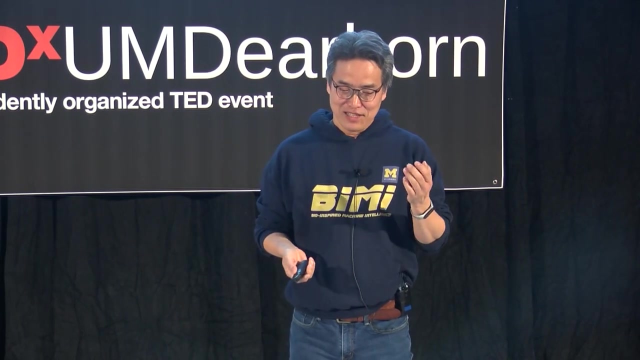 And we have to accept it. should would be OK Not having level 5 in near future, right, It doesn't like imminent emergent thing, like how would I say? like climate change, OK, Like doing now, other than we'll have something catastrophe. 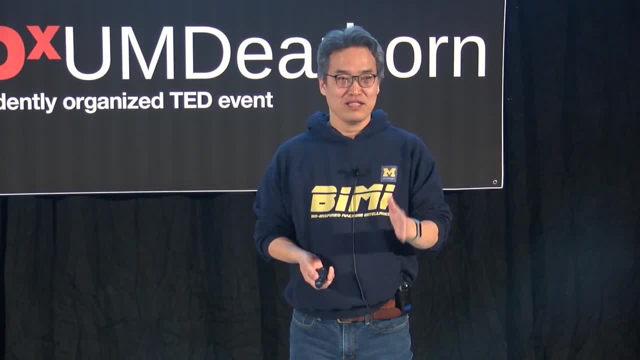 And then the last thing is we have to accept the level 5 is a direction to go, not a goal to reach in a few years. Thank you, Thank you for your attention.